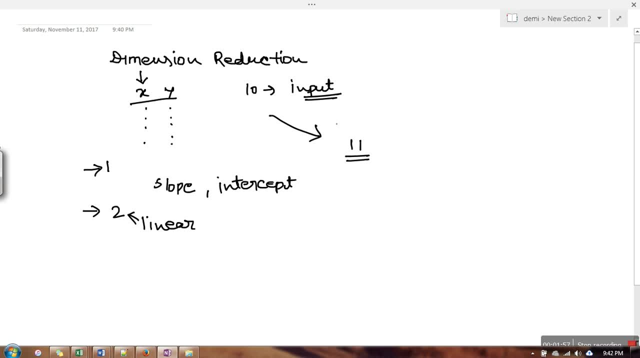 we can say, as the number of dimension increases, the number of parameters for the model also increases. so in our case we have considered only a linear model, which is simple model. so if we start considering other model as well, so the the number of parameter also increase. now, when the dimension increase, we can 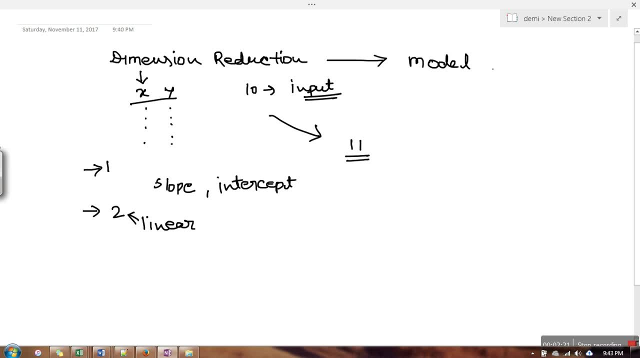 say it will increase model complexity. so how we are going to say that? what is model complexity? so we can consider it as a number of parameter. we need to find out for our model. so in one attributed data we need two parameter for our model. for 10 we need 11. so as we increase the number of 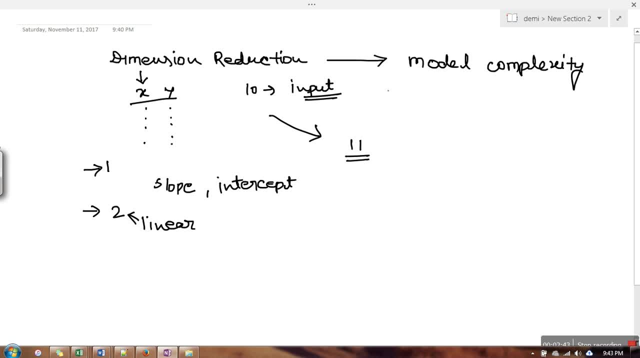 input variable, the number of parameter for our model also will increase. so in simple term, we are saying it: this is the model complexity. so number of dimension- okay, number of dimension will increase model complexity. and what is the another problem if we are having a very high dimension data? let me take this example. 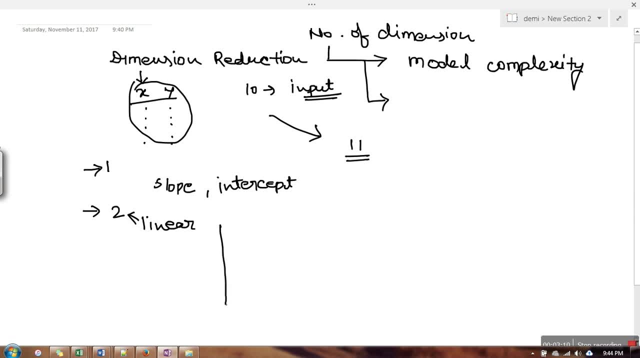 first. so in this example, if this is a regression problem, it means then the type of these values are continuous. so if this is a regression problem, we can plot that data easily. okay. or we can say: we can interpret those data very easily. so if this data is given to us, we can easily see: okay, this is going to. 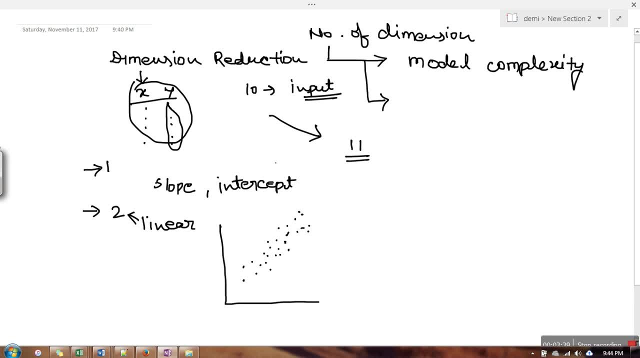 follow a linear trend. but in case, if we are given this data set 10 input attribute, so it will be highly difficult to understand the interpretation of that data. so for high dimension of data, these are the two problem we are having. so first problem: as the dimension increase, model complexity will increase and it also 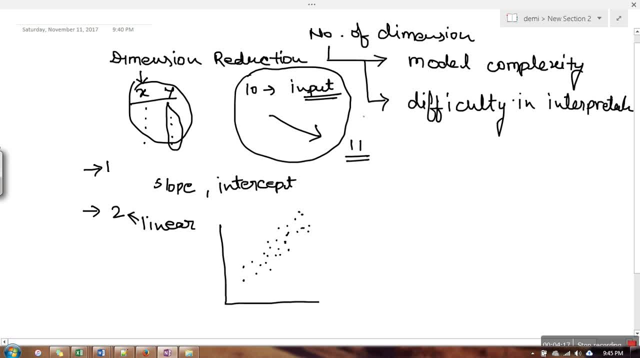 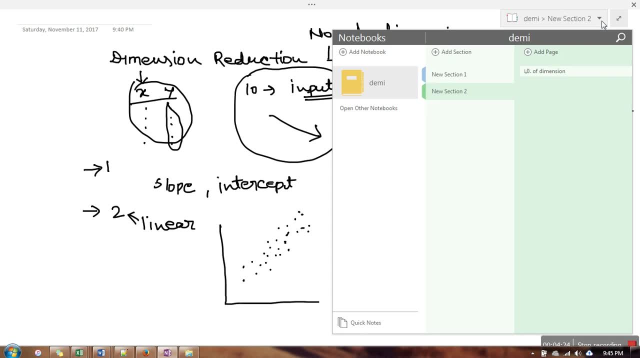 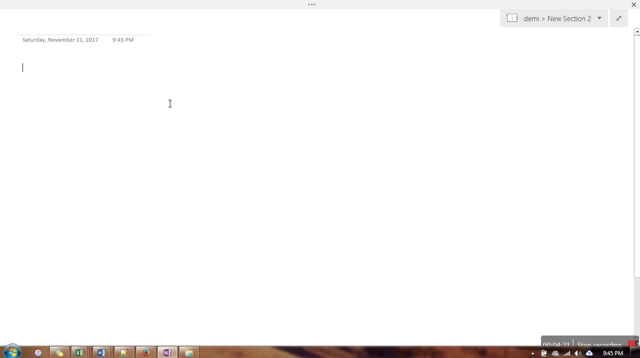 will become difficult to understand interpretation of that data. so, in order to reduce the dimension, principal component analysis is the first method we are going to study now. before going to understand principal component analysis, let me show you some basics, like, let's say, we are given some input. 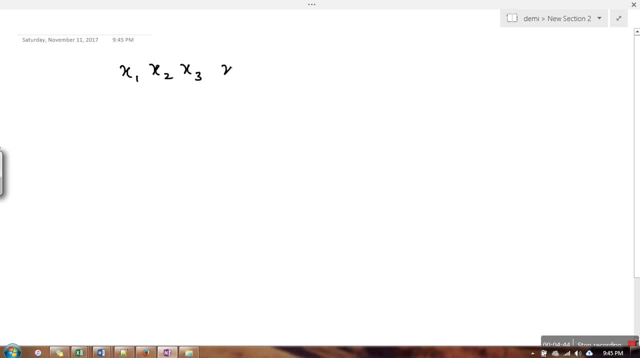 variable x, 1, x 2, x 3 x 4, and this is that target variable. so we are going to. So what people normally do is they usually calculate this entity correlation. Correlation actually tells how two variables are related to each other. 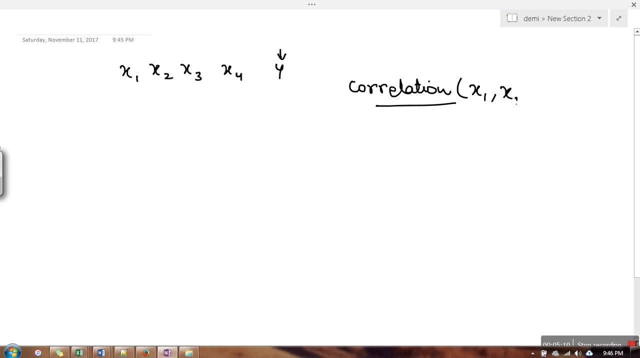 Let me take this example. If for x1 and x2, correlation value is 0.9.. So it means that 90% of the time x1 and x2 variables are relating to each other, Or we can say they are similar to each other. 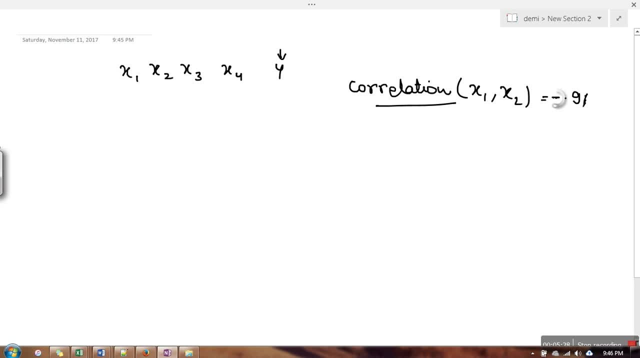 It can be positive, it can be negative. So in case of negative we can say they are negatively correlated. It means if one will increase, another one will decrease. So normally people they calculate the correlation between each pair of these variables. 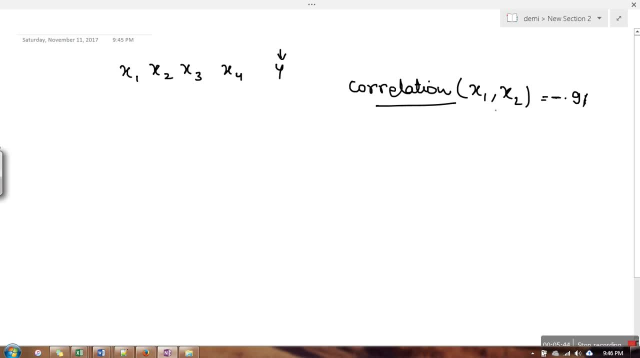 And then they will find out set of pair of variables which are highly correlated. So if a correlation is giving you 0.9, 0.95, it means those variables are highly correlated Or they are conveying same information. 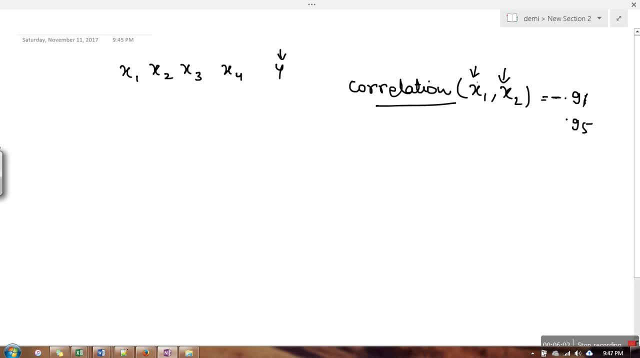 So in that case we can consider only one of them. It will be sufficient. So one way is this of dimension reduction: We can calculate the correlation. So this correlation actually gives us a matrix. So this matrix will be like this one: x1, x2, x3, x4.. 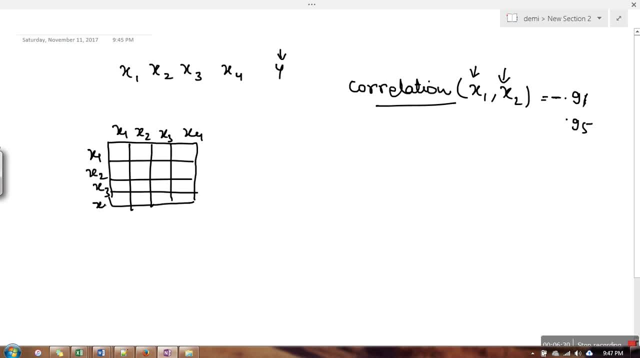 And this side also, So this will be a symmetric matrix, Okay Now. so people normally compute this matrix And on the basis of this matrix, they will decide, okay, which attribute they need to take for their computation. Okay, 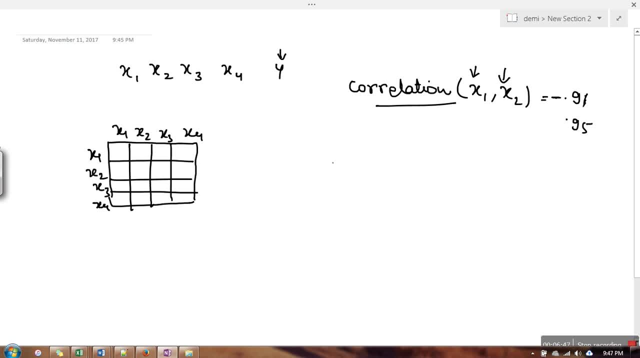 So this is the correlation. Now, next thing is that let me consider a three-dimension data, And in this three-dimension I am having a point, And this point is actually 3,, 4, and 5.. 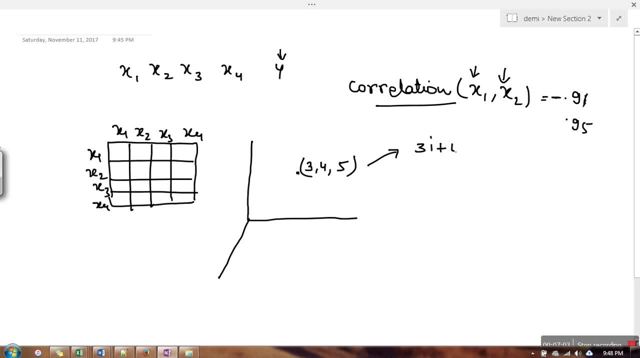 Or in another word I can say it is 3i, 4j and 5k If I am representing this point in a form of vector. So this is the, let's say, value of Now. if someone asks you what is the value of this vector in the direction of x, 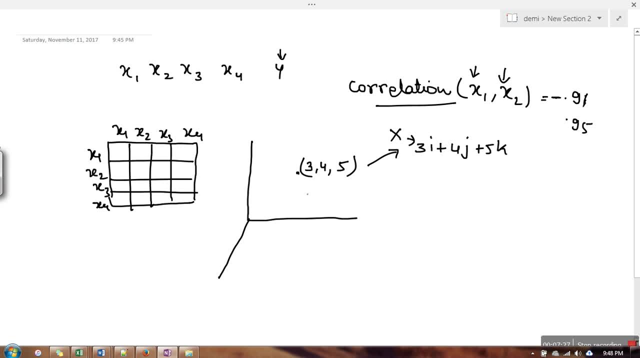 Or in another word, I can say what is the projection of this vector in x direction. So, as we know, in x direction the unit vector is 1, 0, 0.. Or we can say: it is i sorry, i plus 0 plus 0.. 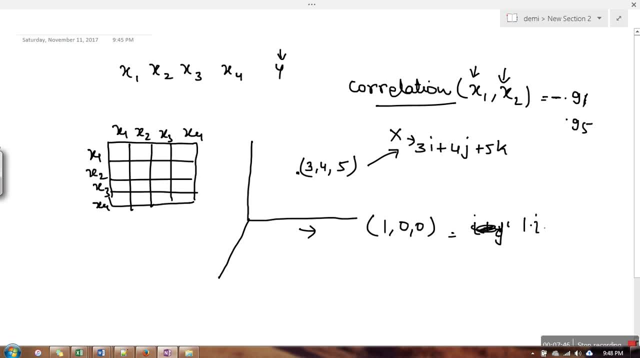 Let me write here: 1 dot i, 0 dot j and 0 dot k. So if we want to find out the projection of this vector in the direction of x, we can simply perform a dot product between x and this input, x. 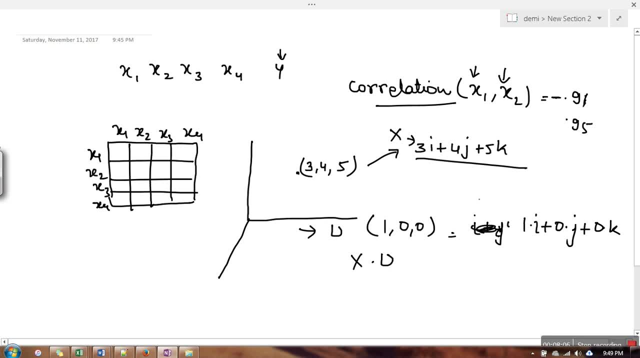 And let's say: this is the direction. u. Now, if we are having these two data in form of matrix, So let's say: this is the, This is the value of x, a vector, And u, which is the direction. this is the direction. 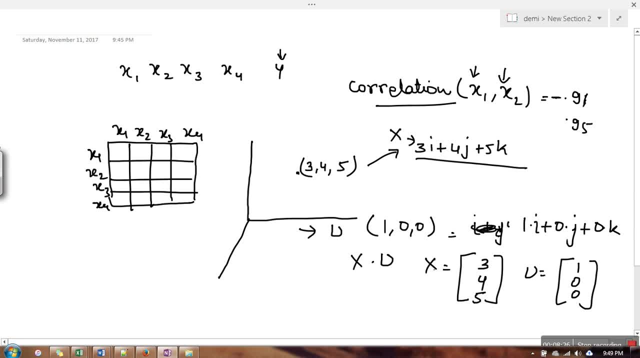 So here, if you want to perform a dot product, what we need to take? We need to take the transpose of this vector or this matrix, And this will take v as it is, So it can be written as xtu. 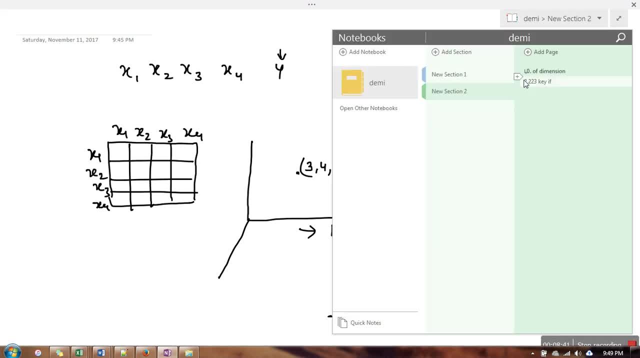 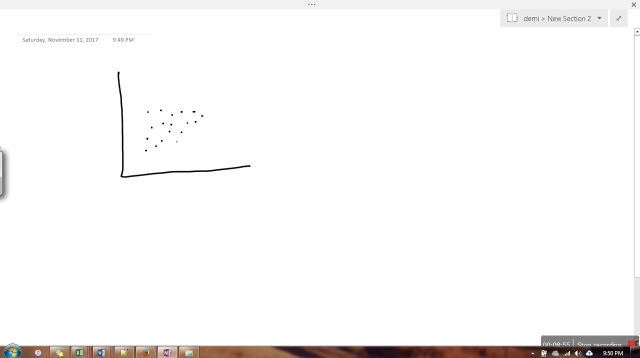 So now I am going to start the principal component. So I am going to start the principal component analysis. So what principal component analysis? say that we are given some data. Okay, now what we have to do. we have to find out in a direction. let's say, this is the direction. I am pointing this direction at you. 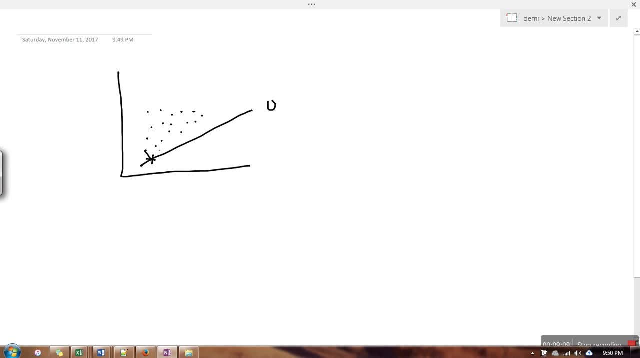 If we project each of these data on this. So what we have to do, we have to find out in a direction. let's say: this is the direction, I am pointing this direction at you. Okay, now, what we have to do, we have to find out in a direction. let's say: this is the direction, I am pointing this direction at you. 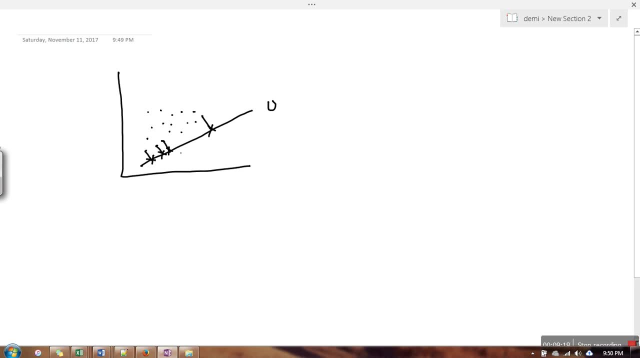 So these are the projected point of these data set. So let's say these are the rest of the data point. So let's say these are the rest of the data point. So the variance of data point will be this one. 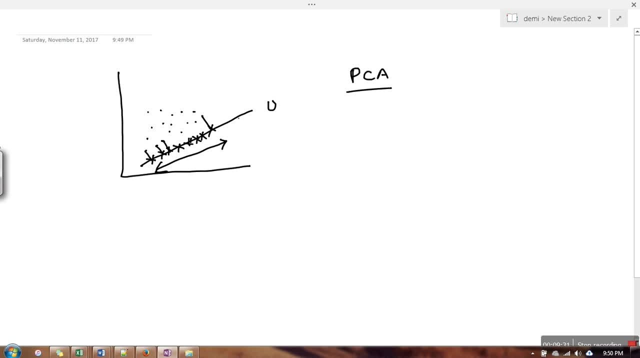 So what PCS says? that find out a direction in which, if we project all of our data, it will give us maximum variance. ok, so this is the core concept of PCA. so what we need to do? we need to find out a direction in which, if we perform, if we project all of our data set and if we 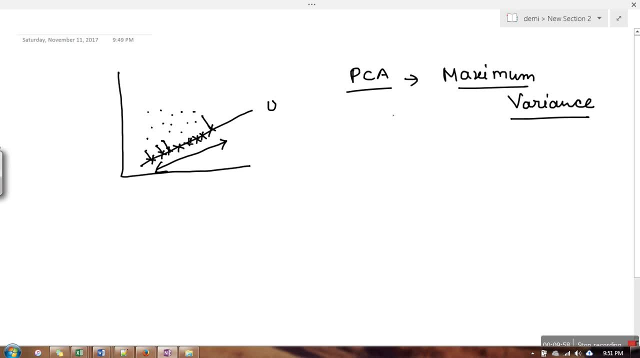 compute the variance, that variance will be maximum. ok, so let's say these data are given in the form of X, ok, and this X is a d-dimensional data and I'm considering this direction as U. so if I want to find out projection of X on U, what I can write, I have to perform dot product and that dot product. 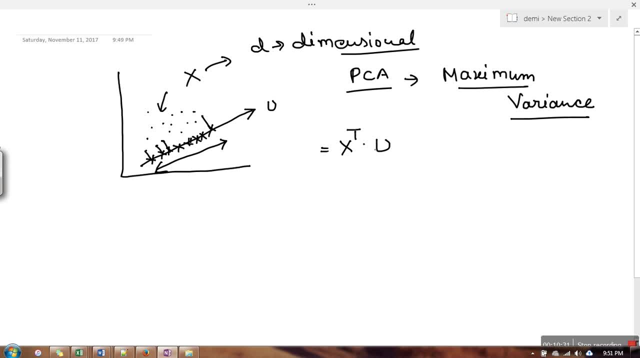 in matrix form can be written as: X du. this is a matrix product and d representing u transpose and I am representing it as a jet. it means jet is these points, that's the z1, z2, z3, z4 and so on. so I am representing all of them by jet. so this: 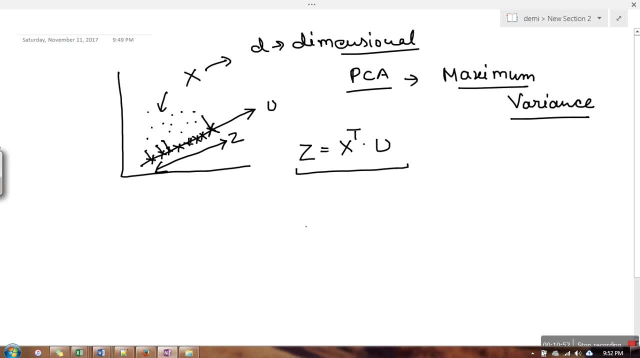 is the projection. ok, now we are making here one assumption. what is that assumption? we are saying that we are considering this data as mean centered data. what is the meaning of mean centered data, considering we are having mean zero, all these data, point. if we consider their mean, it will be 0. so some of us may have might have confused that. 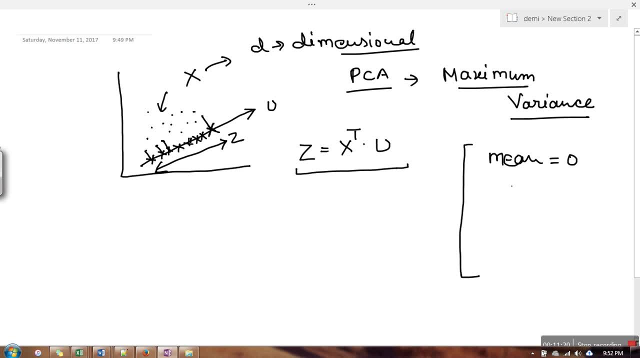 why we are considering this one or this is not the situation with all of our data. so what we can do, we can. we can go to a data, a mean, centered data, by using this formula. so if we subtract mean from each data point, we will whatever data point we 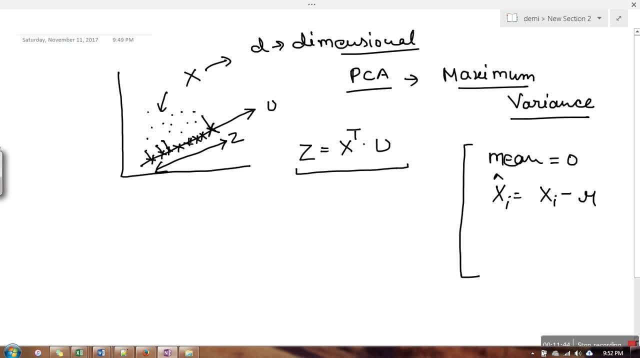 will get. mean of those data points will be zero. okay, so this is our assumption. in case, if this is not true, we can convert our data into mean centered data. now, so here, these all data points are z1, z2, z3 and so on. now we want to. 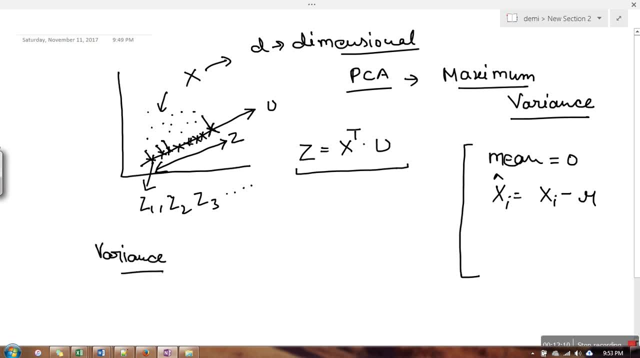 find out variance of this data and, as we know, variance. what is the variance? variance is actually. we are given some data in form of x1, x2, x3. the variance actually x, y minus mu, 1 upon n. summation: okay, so this is the variance, so we will apply the same. 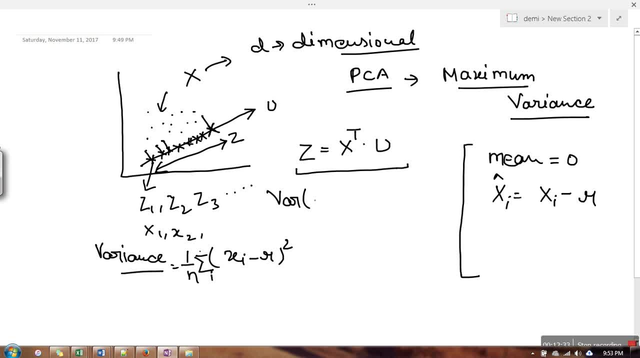 formula here and we want, we will try to compute the variance of jet. so here we have considered mean of our data: 0. so therefore here I want to compute the mean of jet so I can write this mean as this form. okay, now let's put value of ZI here, so value of ZI here will be. 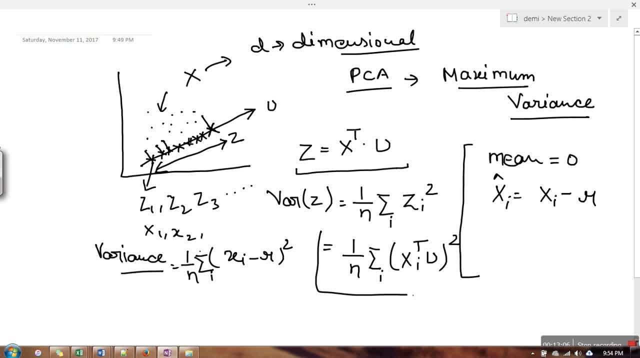 okay, so we got this. now we are having some vectors. that's a vector is our x1, x2, x3, and I want to perform x2. what is x2, x2 is x1, square, x2, square, x3. okay, so, in order to perform x2, which is equivalent to this one, what I can do I can, sorry, I. 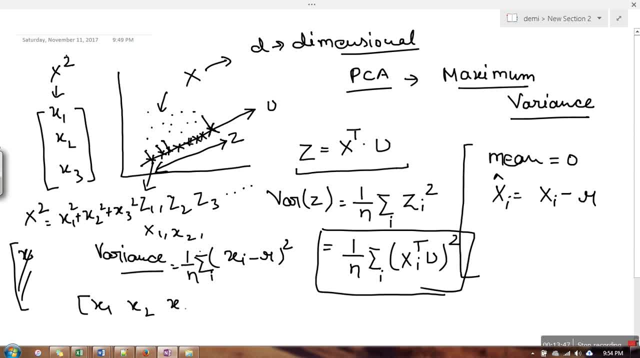 can multiply x1, x2, x3, this matrix, with this matrix, so it will give you the same term. so in another word, I can say: I want to compute the square and if X is in the form of matrix, so I can write it as a X. 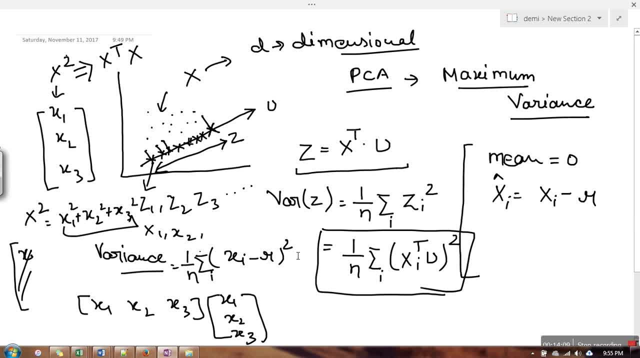 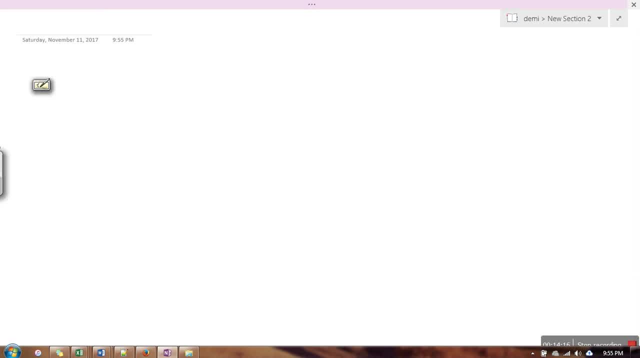 transpose X. but let me take another page. so the quantity we got, that quantity was 1 upon n. I get I square, and we put here our value, and square, in matrix form, can be written as X, I the transpose, U the transpose, and then this one is the simple term. now, if we take this transpose inside, what we will get. 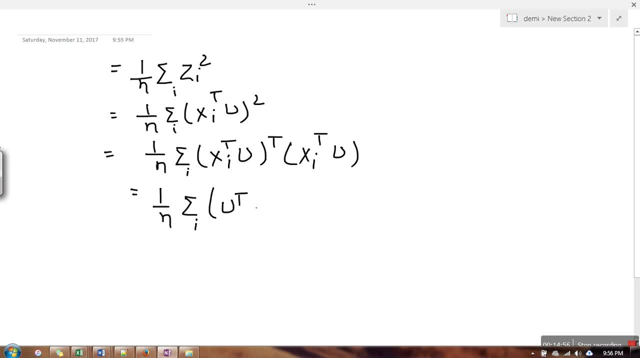 is, we will get U, transpose X, I, so transpose of transpose will be the original matrix and when we take a transpose inside, the order of the inner matrix will be reversed. and this is our rest of the part. so here I can write this one: this is the transpose U, and let me take this summation inside, as you can see. 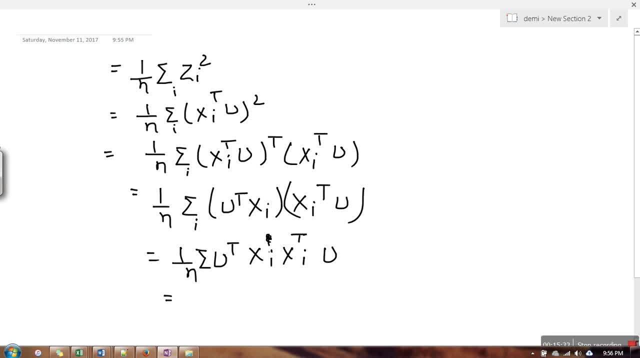 these U are not having any, I okay, so only changing part in this one so I can write this as okay. Now, what is this entity? ok, so let's see, if we are given some X I and this X i is x 1, x 2, x 3, and if we perform, 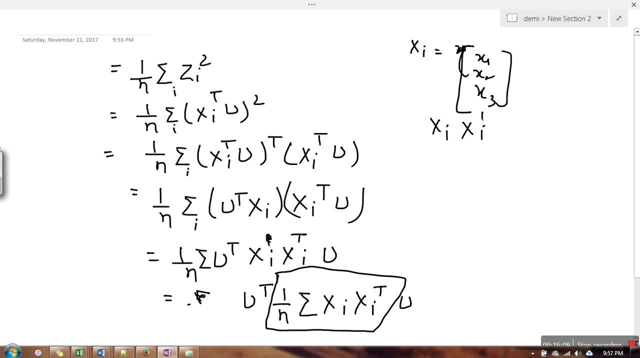 X, I multiply with x- IT, so we are performing product of these two. so if we perform a product of these two, what we will get? we will get a 3 by 3 matrix and this is the summation of all of those matrix and divided by m. okay, so this is actually. 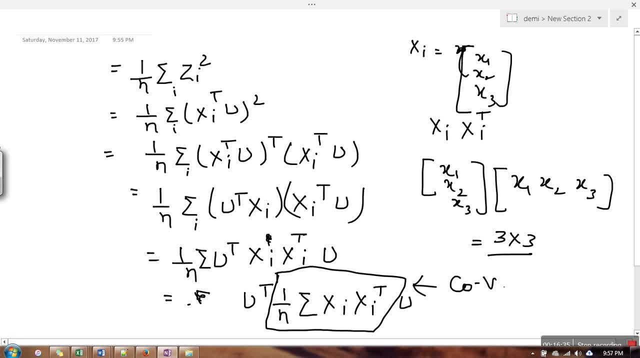 a covariance matrix, okay, and covariance matrix we can denote with summation sign. so what? the term we got? we got this. one variance of Z is equal to UT covariance matrix. and Q- okay, we got this. is the variance after projection. now what is the core concept of PCA? for concept is: we want to maximize this. 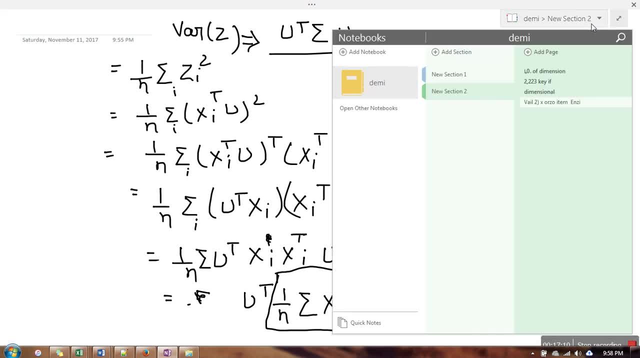 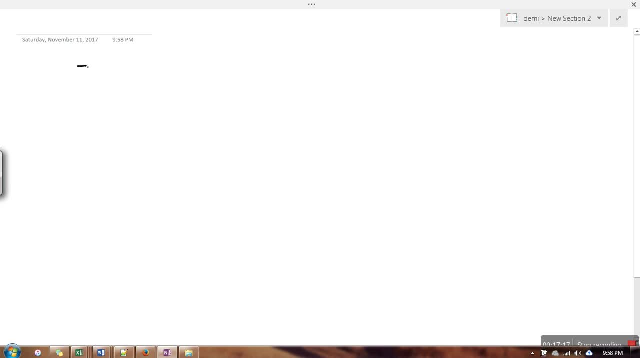 variance. so we want to maximize this variance. okay. now the thing is that田 & У d directions ok, and we are. we will put one more constraint: that u is the unit vector. so if u is a unit vector in another term we can say u square will be. 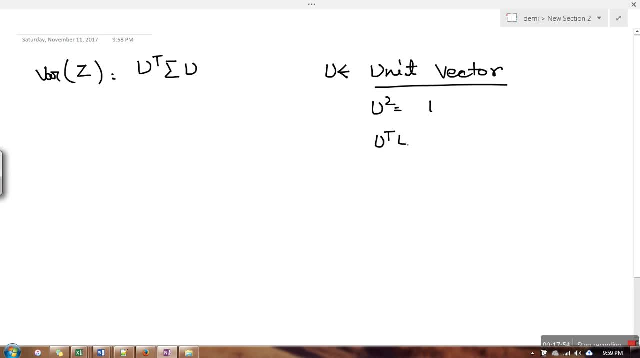 1, and in matrix form, we know what is u square, u square is ut u equal to 1. so now what we are going to do? we are going to combine this expression and this expression into a single problem, and here this is. it can be done by using: 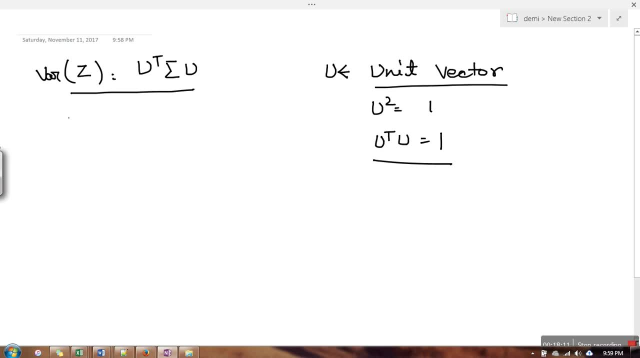 Langrass. so this problem can be written as the language problem. so the final expression we will get, the final expression will be something like this: ok, this is the expression, final expression. so let's say this expression is given to you and the person is asking you have to find out value of you that maximize this. 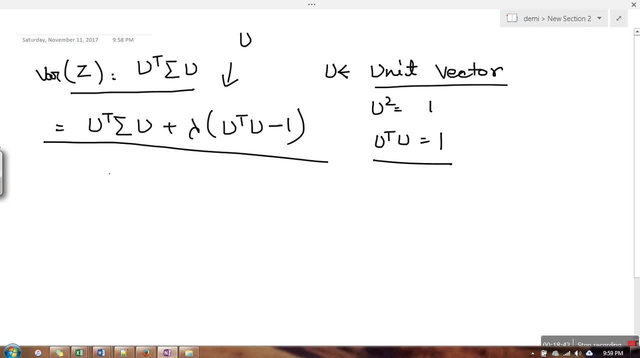 final expression. so here we will use maxima, it will, we will consider it as a maximum problem. so how we used to solve these kind of problem, we will find out the derivative, partial derivative, of this expression with respect to you. so let's say, if I am denoting this as a W, it will be P, w1 and P. so we are going to. 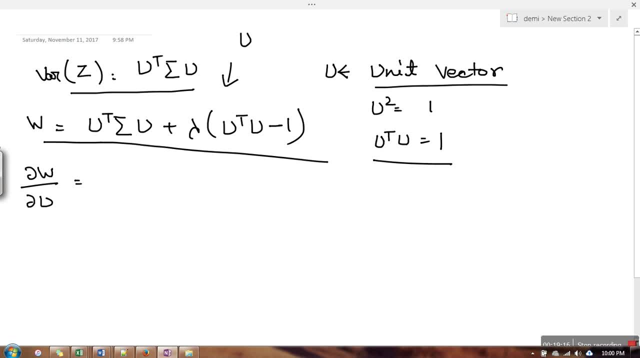 perform the derivation. sorry, differentiation, sorry, I'm sorry. I use the derivation, so we are going to differentiate this term. so first we will perform differentiation on this term. so this is actually u square. okay, we will consider for simplicity, at a u square, and if we perform the differentiation with respect to you, what we will get, we will get to. 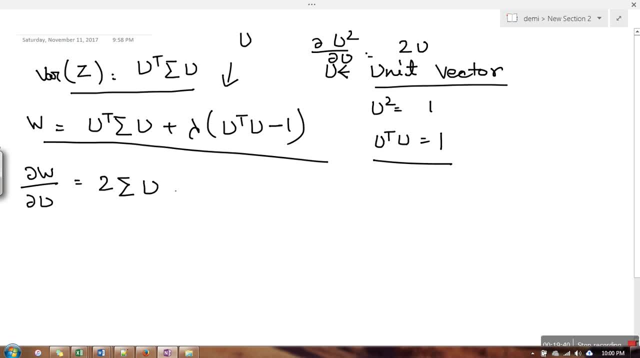 you. so I'm going to write it as a this manner here: what we will get, this also will be considered u square, and if we perform the differentiation, we will get to you and this will be zero. so we have. we will do it for simplicity, and then, if our wh解 looks like: 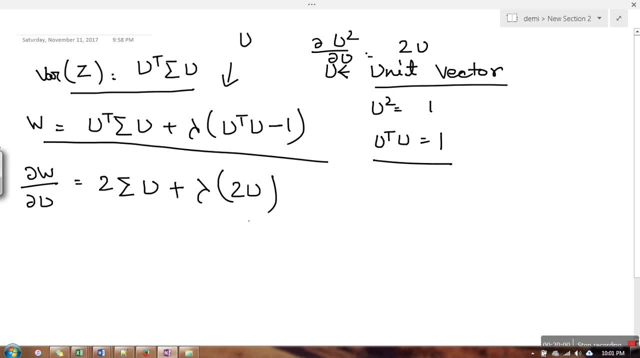 x is equal to 0, then this is our solution of t 2, then this phi is equal to zero. so we have we to find out the differentiation of this term. now we will put it equal to zero and then we try to find out the value of. okay, so from this, 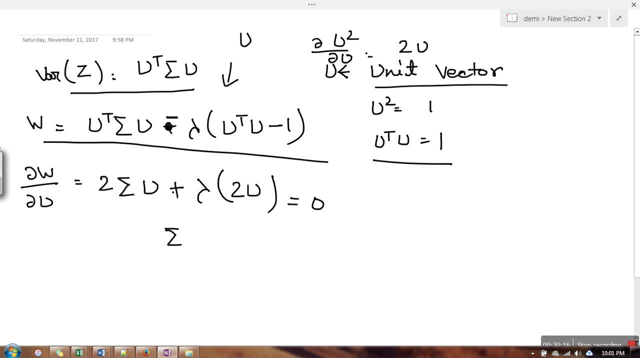 expression. what we actually can't sort for one correction here, this is actually get. is we get this term now here? this is a covariance matrix, this is the unit vector, or direction, this is some constant and this is the same vector, again the same unit vector. so if you can think of this expression, you might have. 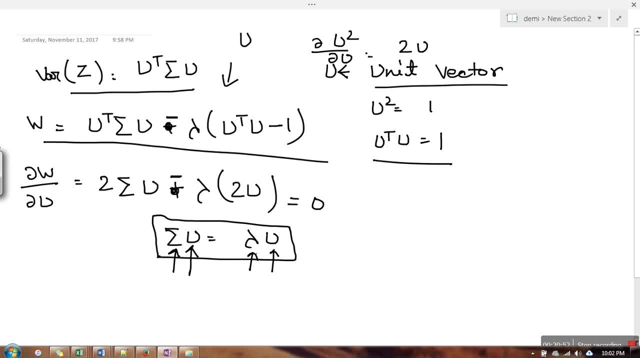 seen this expression somewhere, so it is actually a eigenvector. okay, so u is actually a eigenvector and lambda is here eigen, and this is a very important term. now, what we will do here. we know that variance of Z is a tensor and if we take a square其實 this Högder. 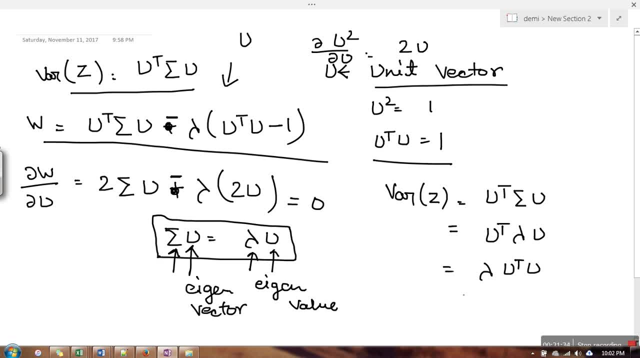 what we are going to work is thenuncer 1äc, department, Part 2. is this something that we will calculate? a actualoriginal mean function for this? Naته propọi, from here we know that the multiplication of these two time equal to Aanda and you, and this become you to you. and, as we know, U is a unit vector and this term is equal to you, square, which is 1. so variance of Z, what is This one? this is actually a eigenvector missing. 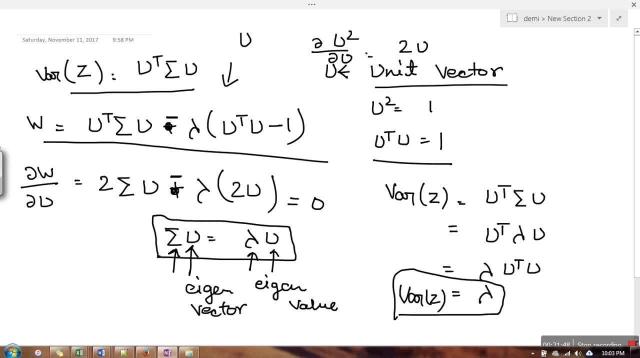 the posição. this one is Torah square. this is stable, so variance of Z is hive. so what is that? this Lemon is constant minus. I should be equal to tau nucleus layers and layer. what is this one? this is actually a eigenvalue. so what? PCA want? PCA want. 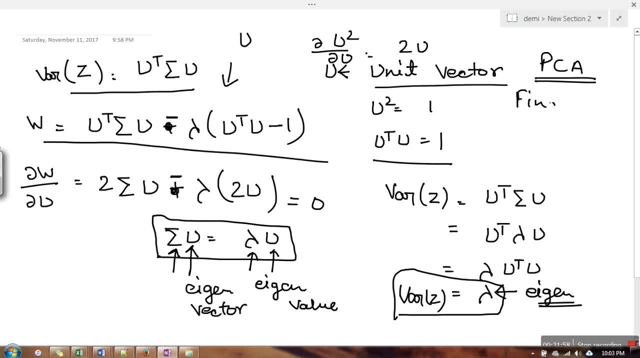 that you need to find, find you such a way that it give maximum variance. okay. and from here we know that variance of Z is equal to eigenvalue. so if we want to find out the maximum variance, that will be the highest eigenvalue of the covariance matrix. so the direction, how we can find out the direction. so 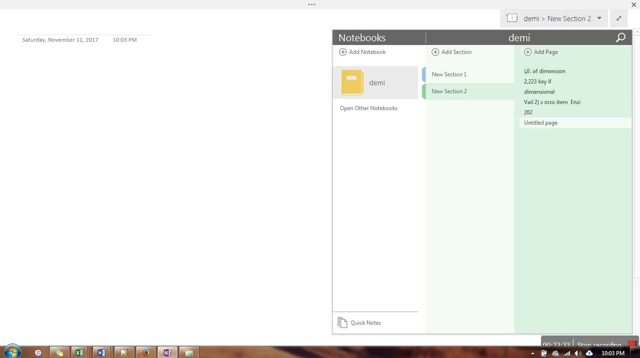 direction. we can find out by finding out the eigenvector of the covariance matrix. so it can be written as: find out eigenvector of covariance matrix. that's it okay, so now. so if you want to reduce our d dimension data to one dimension, what we can do, we can perform, we can find out the eigenvector.